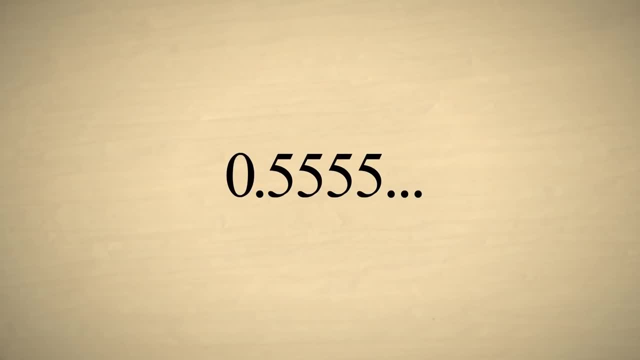 into a fraction. The first step is to eliminate the infinitely repeating digit. We do this by first multiplying the number by ten to shift it one column to the left, and then subtracting the original number, Since both numbers in this example have an infinite number of repeating fives. 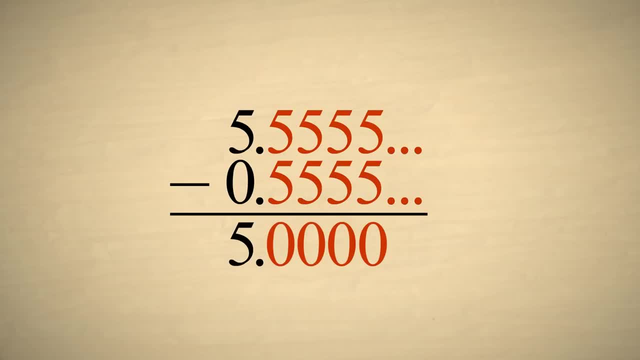 this eliminates all the repeating fives after the decimal point. We know that our original decimal number is equal to some fraction, but we don't yet know what that fraction is. However, we do know that when it is subtracted from ten times itself, we get five. 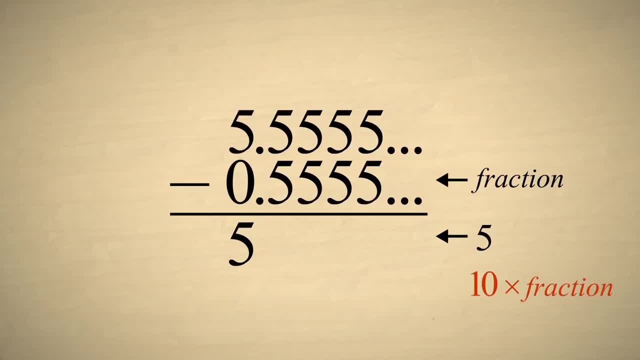 Let's write this statement as an equation: Ten times the fraction minus the fraction equals five. It is possible to write this statement more simply: Subtracting one thing from ten things leaves nine things. So instead of writing ten times the fraction minus the fraction, 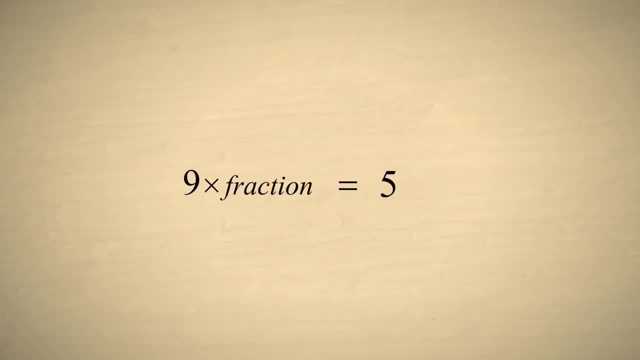 we can simply write nine times the fraction. Since both sides of the equation are equal, we can divide each side by the same number and they will still be equal. Let's divide both sides by nine. Notice that on the left side of the equation, the fraction is multiplied and divided by nine. 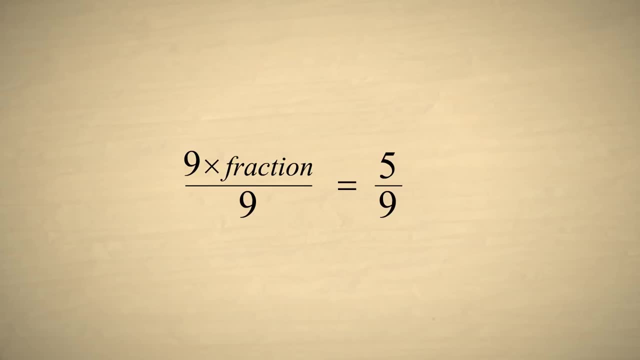 This leaves its value unchanged, so we can cancel out the nines on the left side of the equation. We are left with an equation which says that the fraction is equal to five-ninths. We have converted our repeating decimal number to the fraction five-ninths. 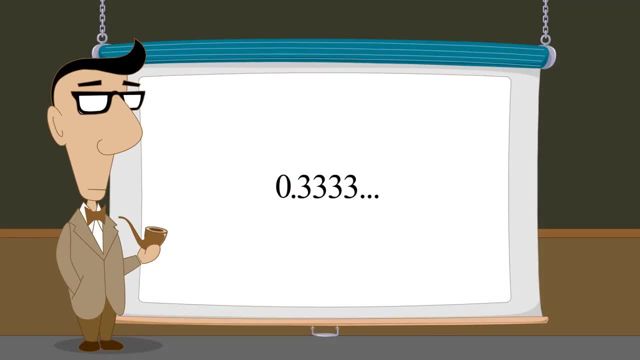 Let's try this again with a repeating sequence of threes, As we did in the previous example. we eliminate the ones that are equal to five-ninths. Let's try this again with a repeating sequence of threes, As we did in the previous example. we eliminate the ones that are equal to five-ninths. 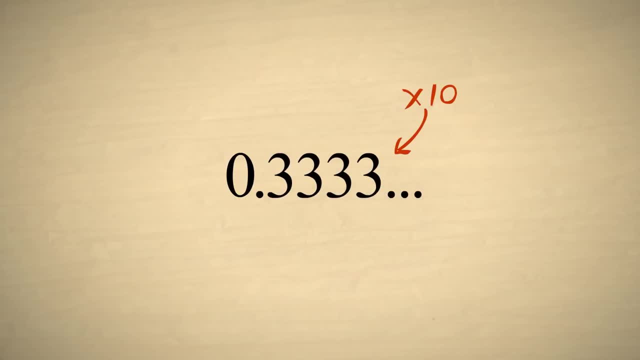 We add one repeating digit by multiplying by ten one time and then subtracting the original number. This eliminates all the repeating threes to the right of the decimal point. So ten times the fraction minus the fraction equals three. We write this as an equation which we can simplify to say: 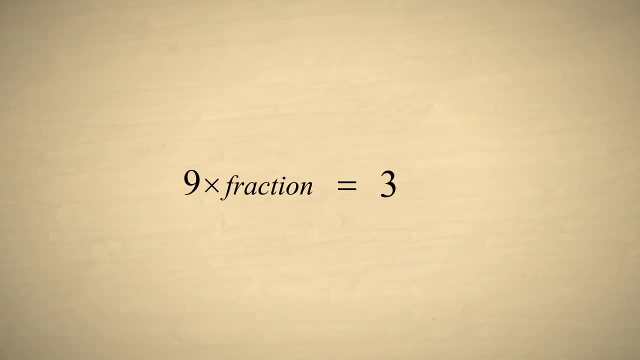 nine times the fraction equals three. We then divide each side of the equation by nine so that the nines on the left side cancel. This equation tells us that our fraction is equal to three-ninths. Of course, the fraction three-ninths can be reduced to one-third. 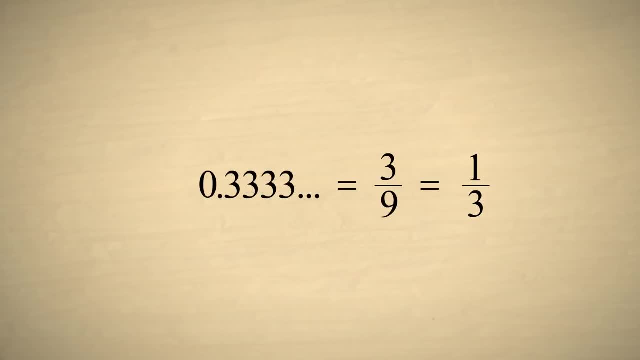 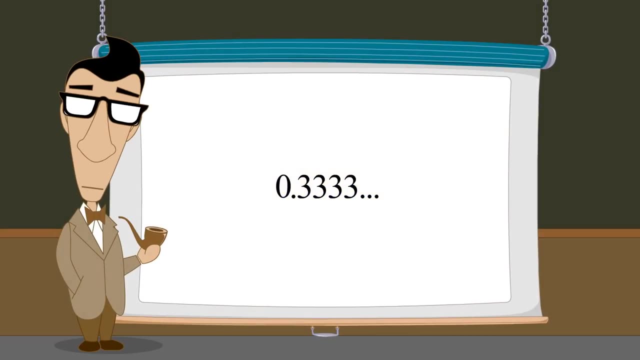 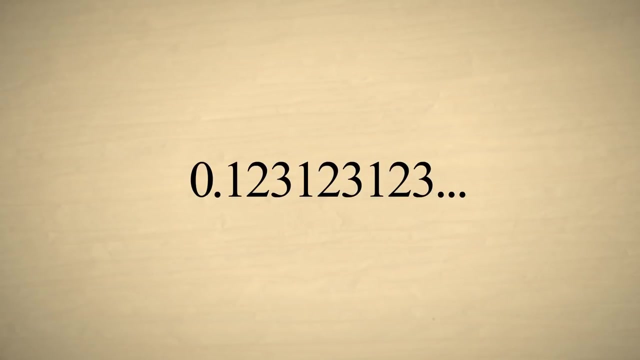 so we have converted this repeating decimal number to the fraction one-third. Now, instead of a single repeating digit, let's convert a decimal number with a repeating sequence of three digits. Since there are three repeating digits to eliminate, we must shift the number three columns to the left. 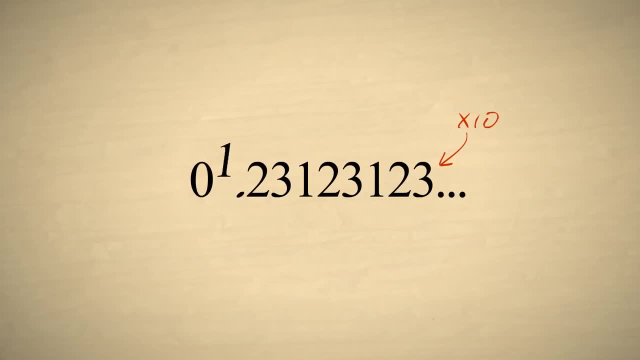 by multiplying it by ten. three times. This, of course, is the same as multiplying by one-thousand. We then subtract our original number, which eliminates the repeating digits. Now we write this as an equation: one-thousand times the fraction minus the fraction equals one-hundred twenty-three. 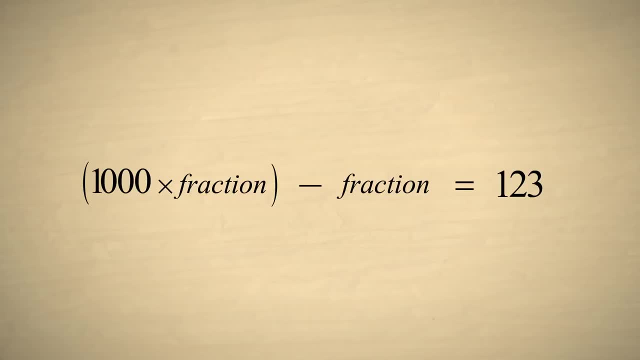 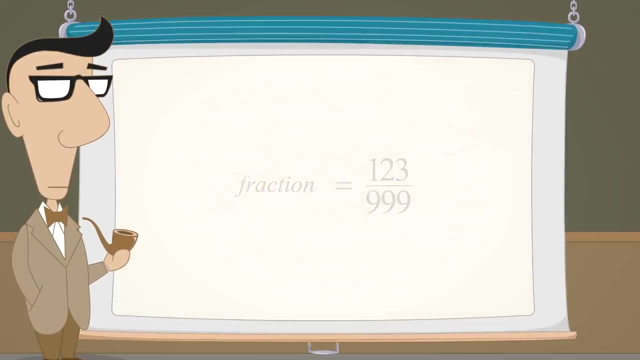 One-thousand times the fraction minus the fraction is the same as nine-hundred ninety-nine times the fraction, And dividing both sides of the equation by nine-hundred ninety-nine cancels out the nine-hundred ninety-nine on the left, so our fraction is equal to one-hundred twenty-three nine-hundred ninety-ninths. 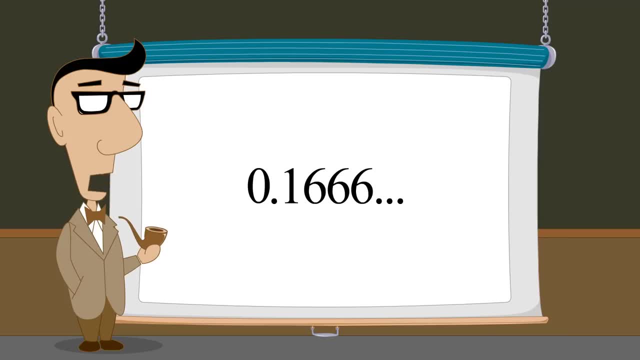 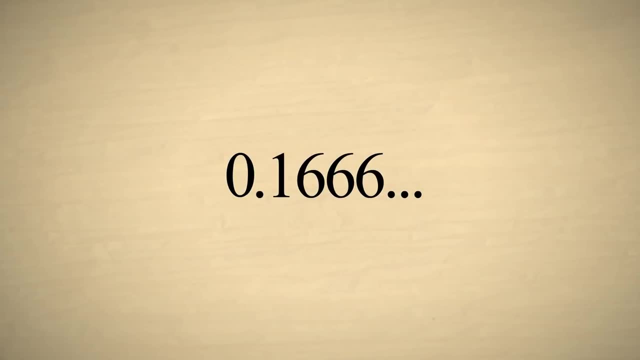 Let's see what happens with the repeating decimal number zero point one, followed by an infinite number of sixes. Since there is only one repeating digit, six, we shift the number one column to the left by multiplying by ten one time And subtract the original number. 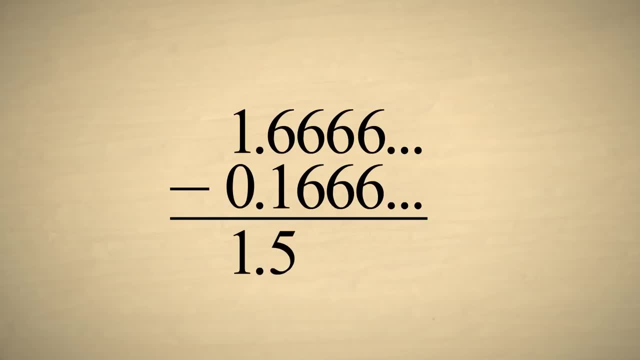 This eliminates the repeating sixes and we are left with one point five. We then write the equation: ten times the fraction minus the fraction equals one point five, which we can simplify to nine times the fraction equals one point five. Dividing both sides of the equation by nine eliminates the nines on the left. 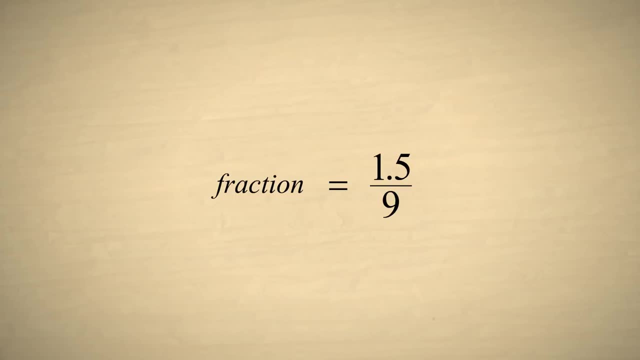 And we see that our fraction is equal to one point five over nine. But we have a problem: A fraction's numerator and denominator must be integers. We can solve this problem by multiplying the top and bottom of the fraction by ten to create two integers. 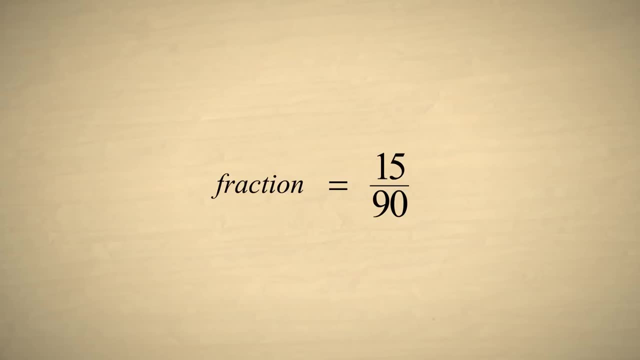 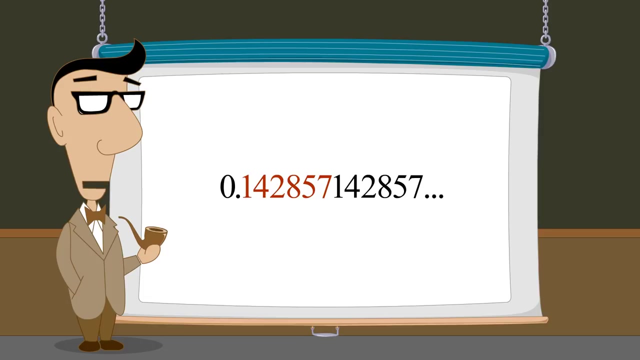 This gives us fifteen-ninetieths, which can be reduced to one-sixth, So this repeating decimal number is equal to one-sixth. As a final example, let's reduce a number that has the repeating sequence of digits one, four, two, eight, five, seven. 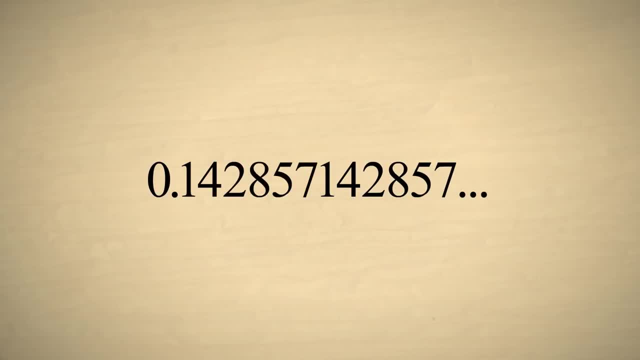 Since there are six repeating digits, we shift this number six columns to the left, by multiplying it by ten, six times, which is the same as multiplying by one million. We then subtract the original number. This eliminates all but one copy of the repeating sequence. We are left with the integer one, four, two, eight, five, seven. 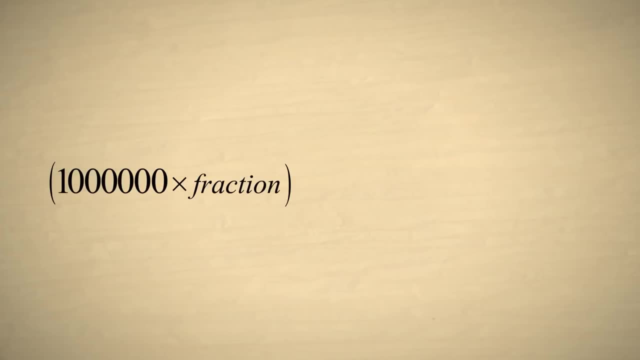 We then write the equation: one million times the fraction minus the fraction equals one, four, two, eight, five, seven. Using the same logic as before, this equation can be simplified to nine, nine, nine, nine, nine, nine times the fraction. 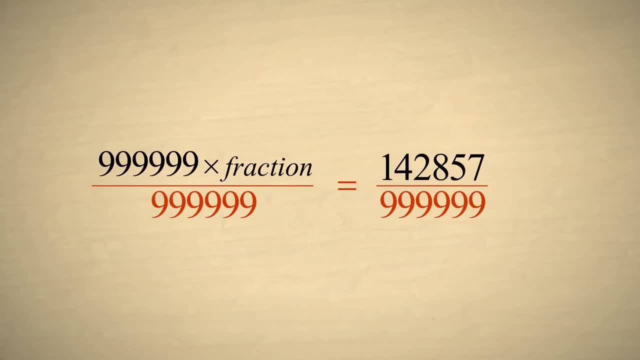 Dividing both sides of the equation by nine, nine, nine, nine, nine, nine leaves us with an equation which says that our number is equal to the fraction one, four, two, eight, five, seven over nine, nine, nine, nine, nine, nine.